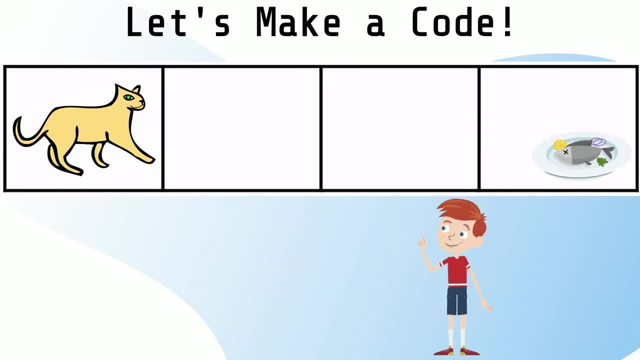 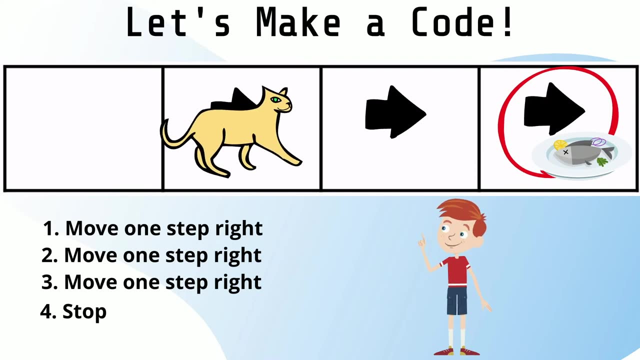 to the right to get her cat food. I will need to code a specific step-by-step set of instructions. This is what my algorithm would look like. I need to tell the computer one step at a time, to help it understand where the cat needs to go. I also need to make sure I tell the computer when to stop or the cat moves past the cat. 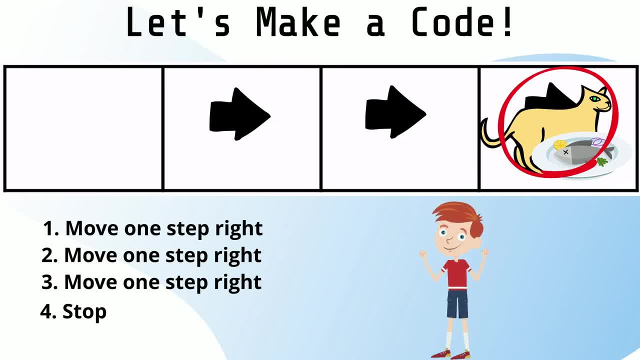 food. Also, I want to know the right and wrong selecutive process for ‑‑. okay, so I have to put the computer at reading limit. remember, without moving down one box, one box, as that cat goes to a was able to use code to write an algorithm. This algorithm told the computer to make the cat move. 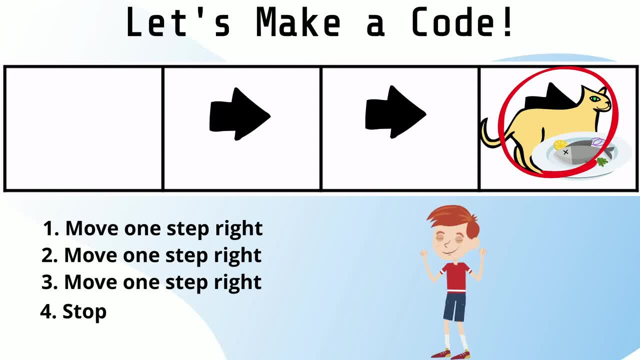 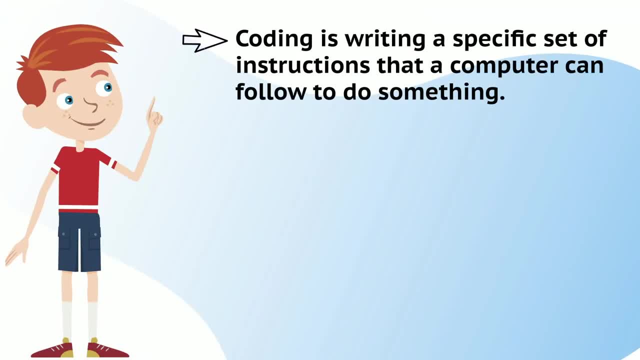 three steps to the right to get her cat food. Okay, let's review what we have learned. Coding is writing, a specific set of instructions that a computer can follow to do something. Computer programs are a finished set of instructions that a computer follows to. 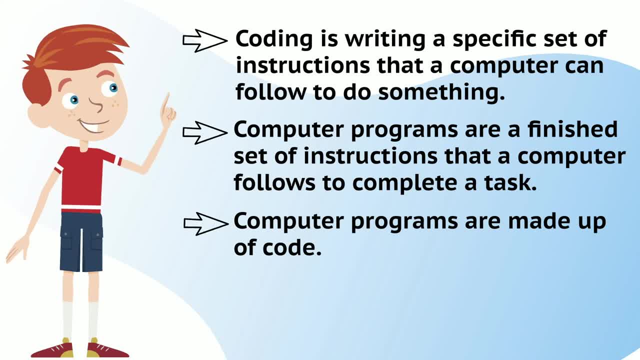 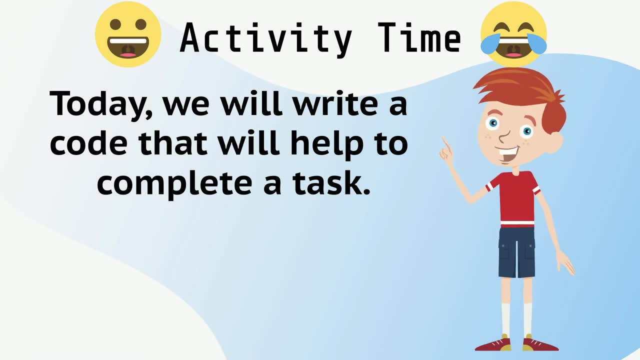 complete a task. Computer programs are made up of code. A code is a step-by-step set of instructions written in a way that a computer can understand: Activity time. Today we will write a code that will help to complete a task. Take a look at the screen. I need an algorithm. 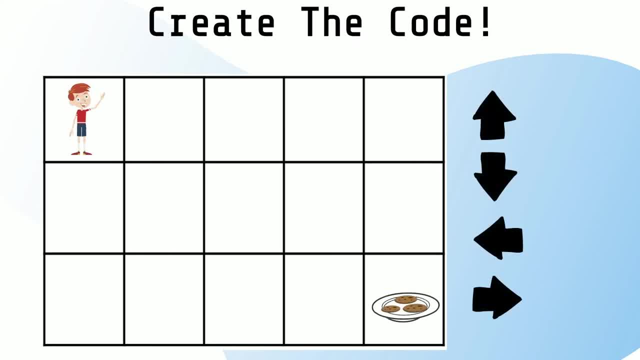 to help me reach my favorite snack. Here are the codes you will need to write the algorithm. I can only move up, down left and right. Can you write an algorithm that will help me reach my favorite snack? Pause the video here to complete your answer. 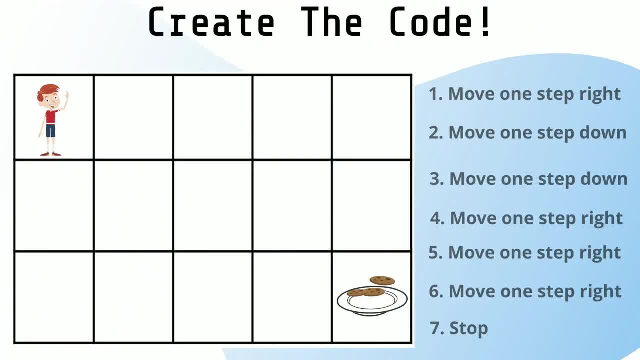 Here is the answer. First, I will need to move one step to the right. Then I will move one step to the left. I need to move two steps down. Next, I will need to move three steps to the right. Finally, I will need to stop. 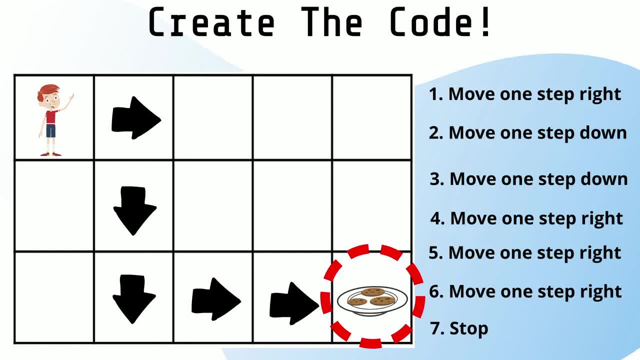 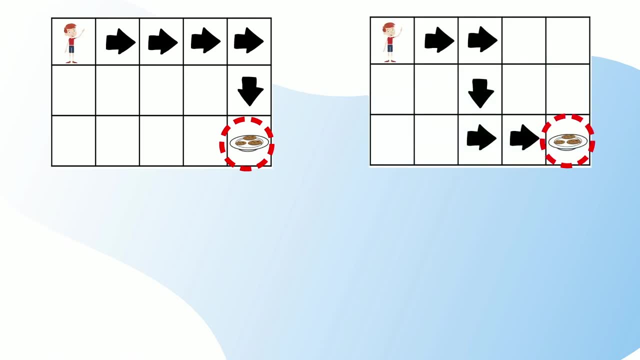 Yay, now I have my cookies. Thank you for writing the code. If your code looks different, that's okay. There are some other codes you can write to help me reach my favorite snack. Here are a few other options. Check your code to see if your answer matches the screen.